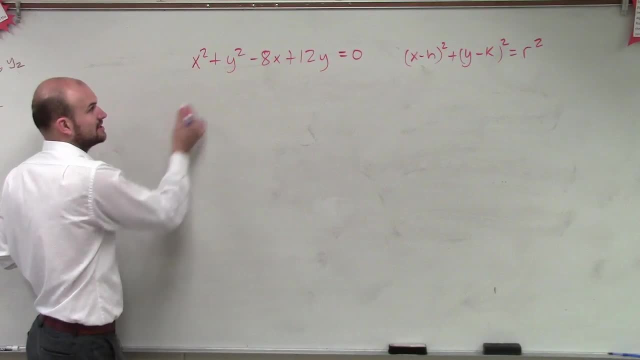 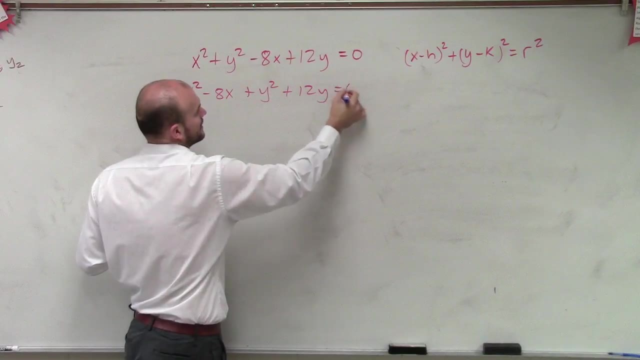 So what we're going to do to complete the square, we first have to arrange our variables together, So we have x squared minus 8x plus y squared plus 12y equals 0.. Now I can complete the square for each of these separately. 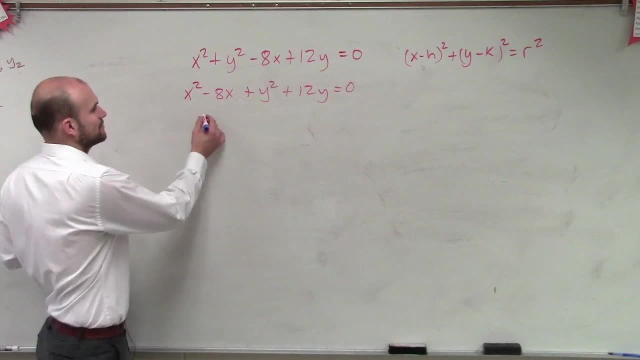 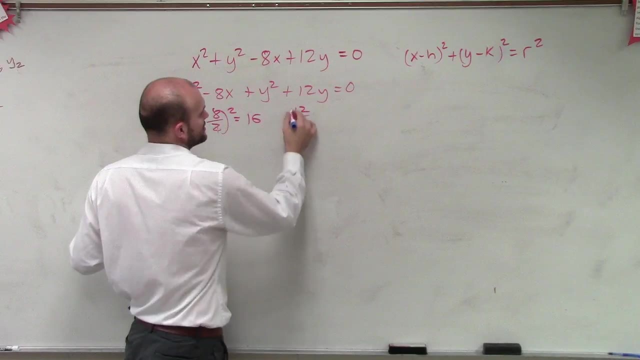 Fortunately for us, we don't have any coefficients, right, So I can just do this one as negative: 8 divided by 2 squared, which equals 16.. This one's, 12 divided by 2 squared, which equals 36.. 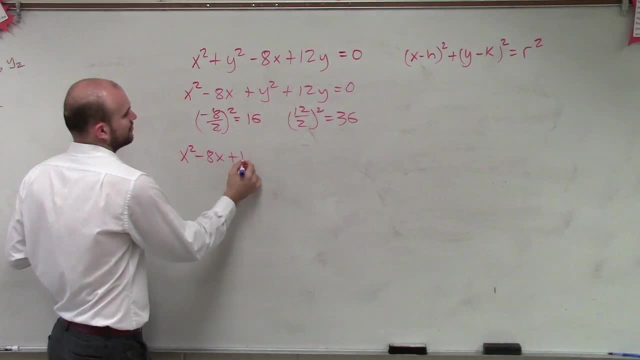 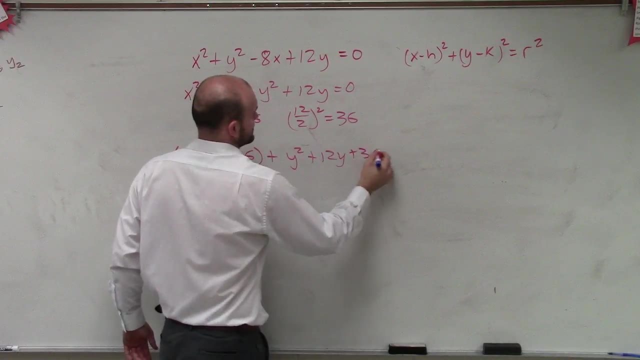 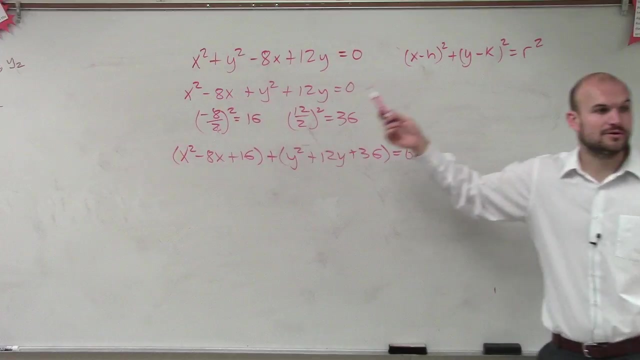 Therefore, I can write this as x squared minus 8x plus 16, plus y squared plus 12y plus 36.. Now remember, since I'm adding a 16, I have to. I could subtract 16 on the same side, but I don't really want anything else. 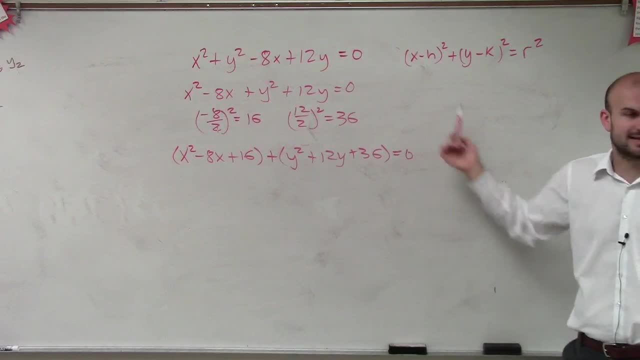 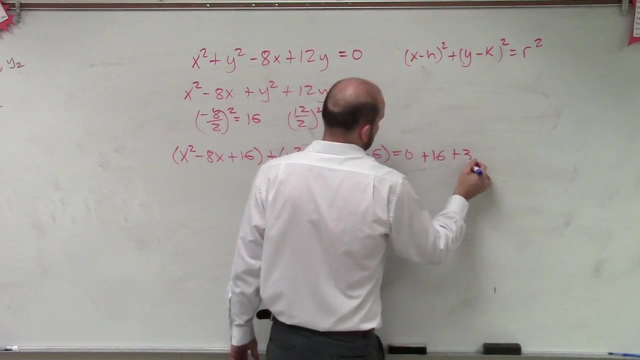 except for my binomial squares on the left side. So I can put it on the other side. So if I add 16 on the right side, I have to add to the other side. All right, Now I can rewrite this as a binomial squared. 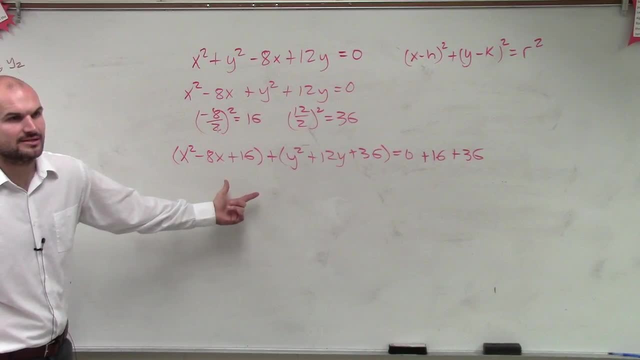 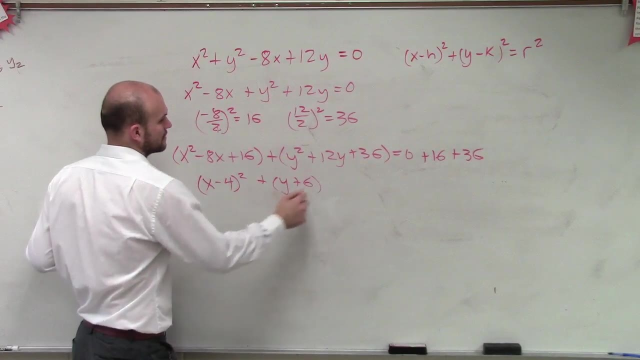 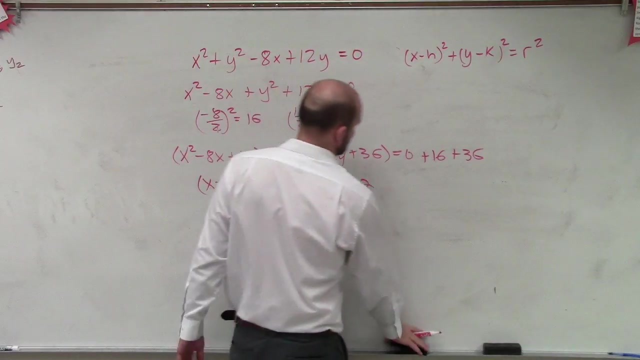 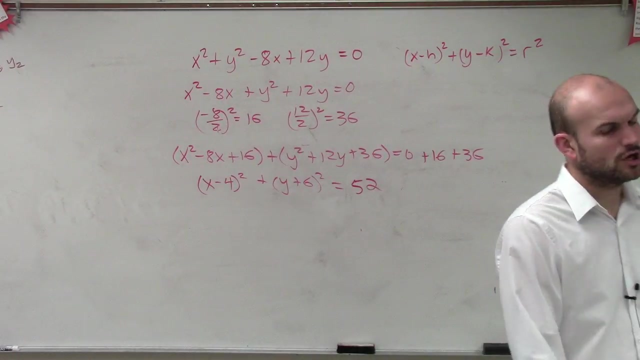 So by factoring this, by factoring this, I write this as: x minus 4 squared plus plus y plus 6 squared equals 42. 52.. Okay, So now we need to determine what is my radius right. Oh crap. 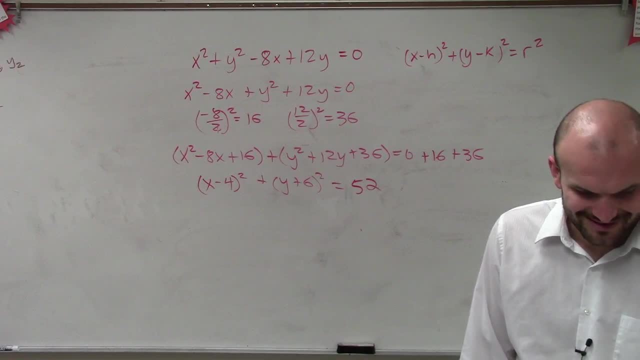 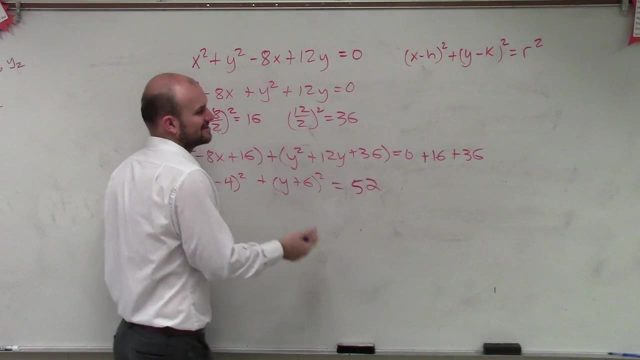 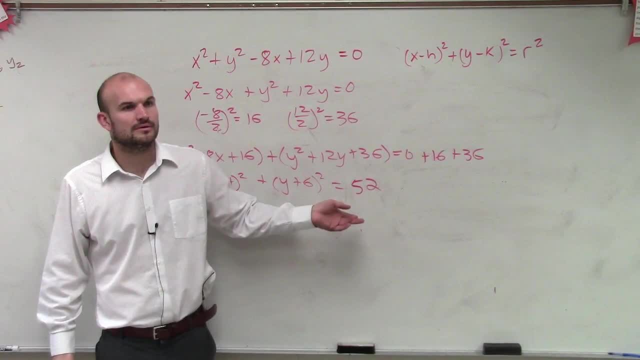 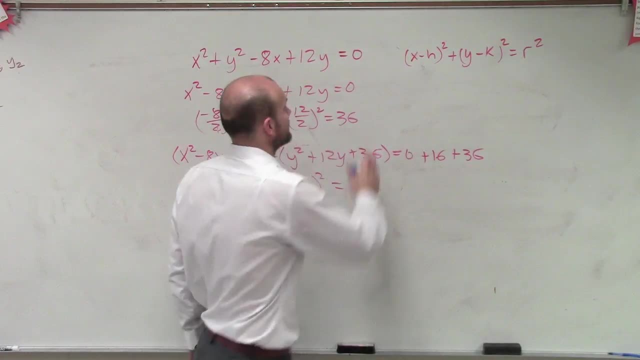 Is it going to be kind of hard to graph a radius when you have it as 52?? Yeah, So let me go and rewrite the problem again that I had. I think I did write this, So it's plus 12 at the end. 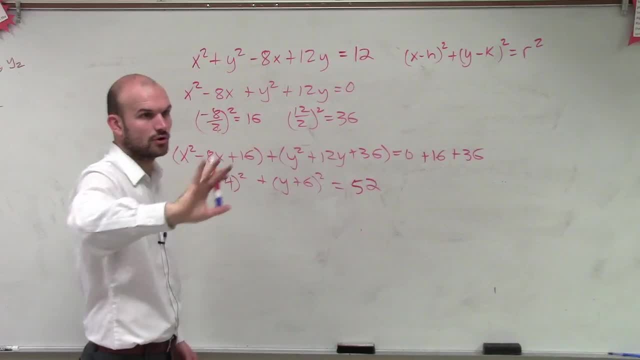 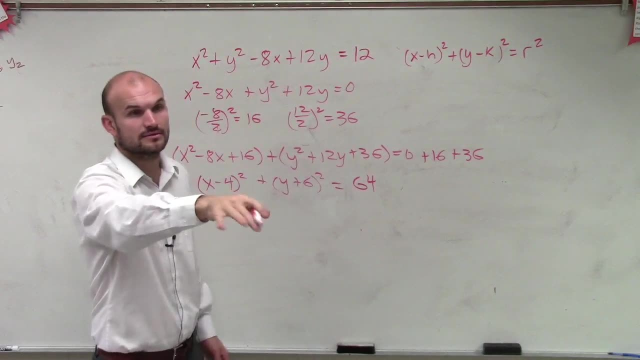 Destin Alex, could you guys find two different seats? Just not even that row, Just totally two different seats. So therefore this ends up equaling 64.. So find two different seats, Not on that row, Anywhere, I don't care.